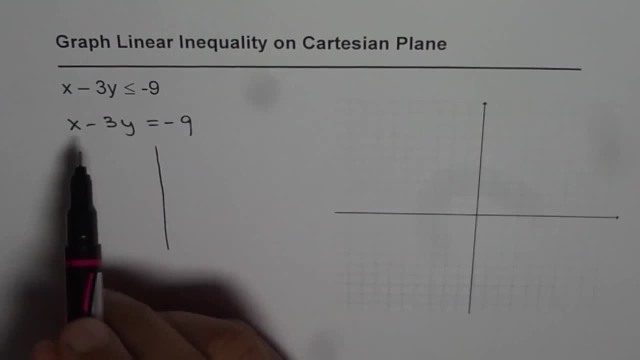 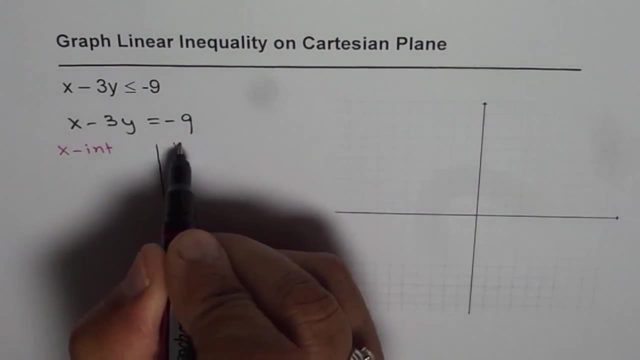 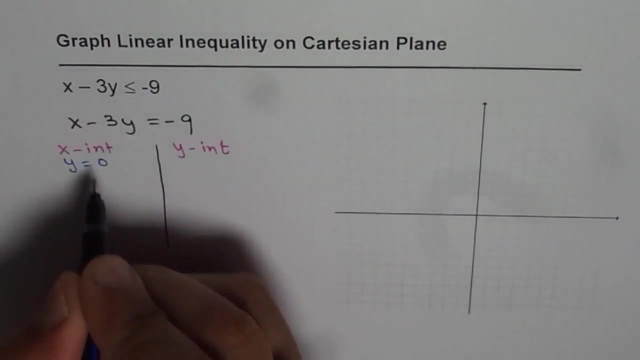 to sketch this line. That is probably the best method When you are given in standard form or a form like this. we should find x intercept And y intercept to sketch the line. So x intercept means y equals to 0, y intercept. 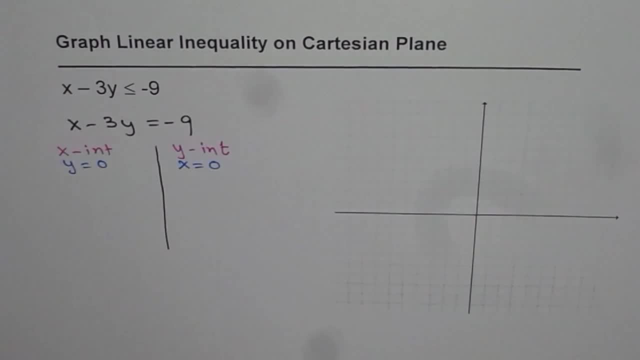 means x equals to 0.. Find the value of y For y intercept. find the value of x for x intercept. So if y equals to 0, that means, if you hide this term, you have got x equals to minus 9.. So you get x equals to minus 9.. So that is your x intercept. So 1,, 2,, 3,, 4,. 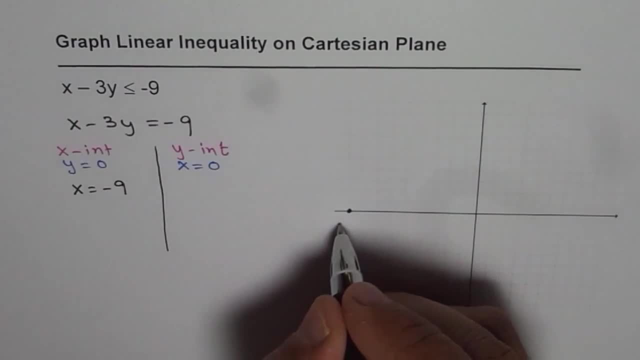 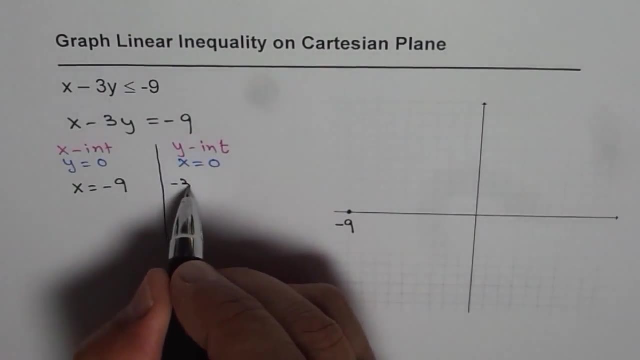 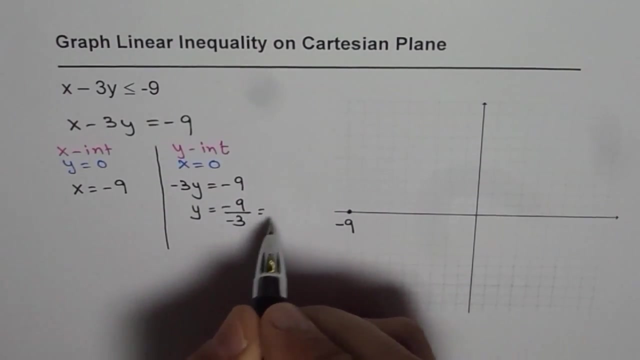 5,, 6,, 7,, 8,, 9.. So that gives you minus 9 x intercept For y intercept, x equals to 0.. So you get minus 3y equals to minus 9, y equals to minus 9 divided by minus 3, which. 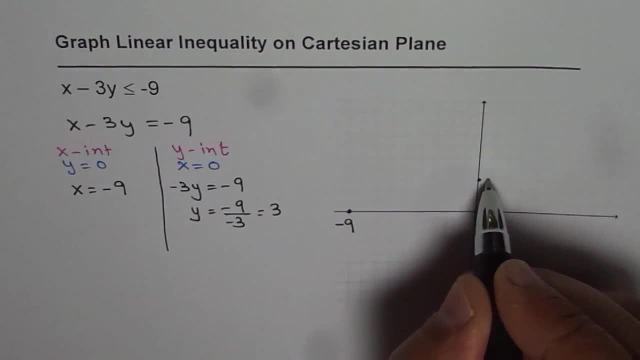 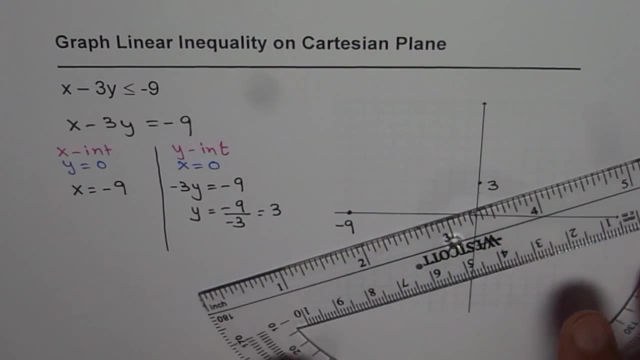 is 3.. So it is 1,, 2,, 3.. That is the y intercept. Now, once you join these two points, you get your line, which is x minus 3y equals to minus 9.. So that is the y intercept. So that: 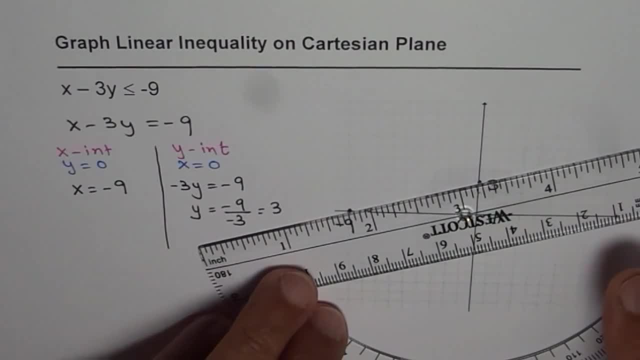 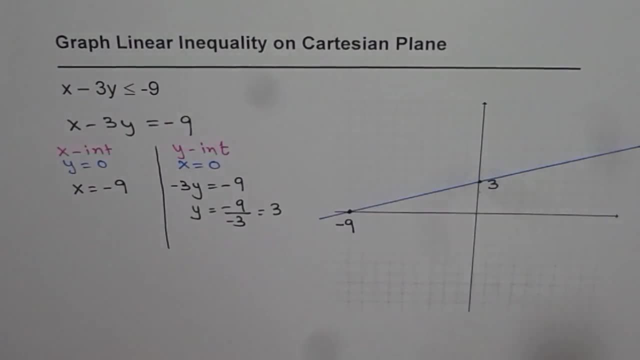 is the line which represents x minus 3y equals to minus 9.. But the question is what? The question is: less than equal to minus 9, correct. Now, less than equal to that means we need to shade something which is either above the line or below this line. 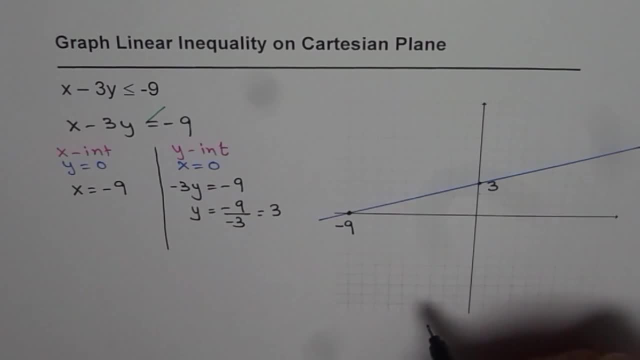 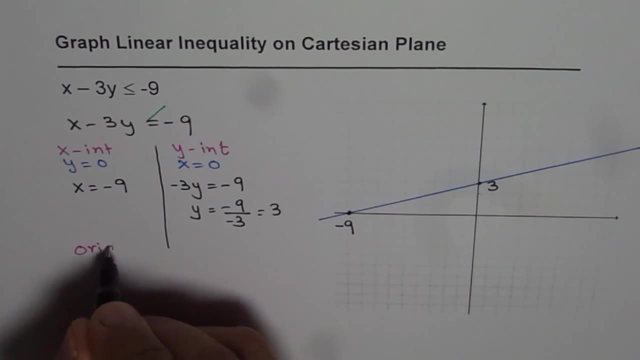 The question is how to figure out which one is the right area For that. what we can do is we will always do the 0 origin test. We will check if origin is in our solution or not, right. So origin test whether it is in the solution or not. So if I write origin, 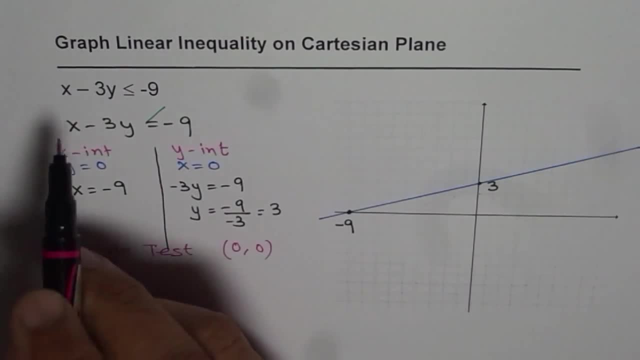 means this point right: 0, 0.. If I write 0, 0, I get 0, 0. So if I write 0, 0, 0, I get 0, 0, 0. So I get 0, 0, 0.. So if I write 0, 0, 0.. So if I write 0, 0, 0, I get 0, 0, 0.